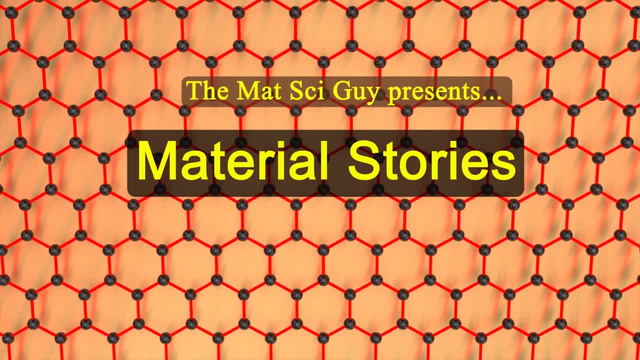 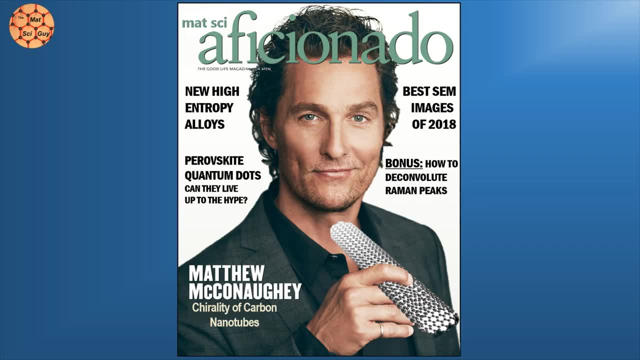 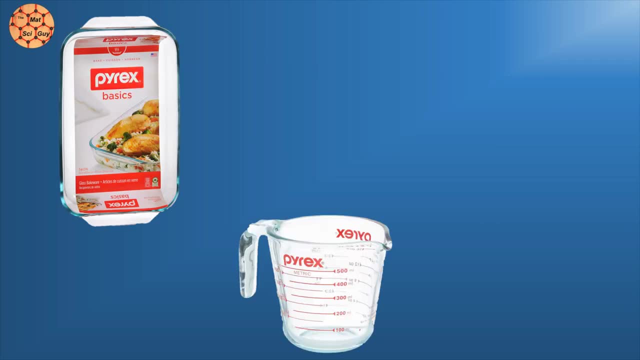 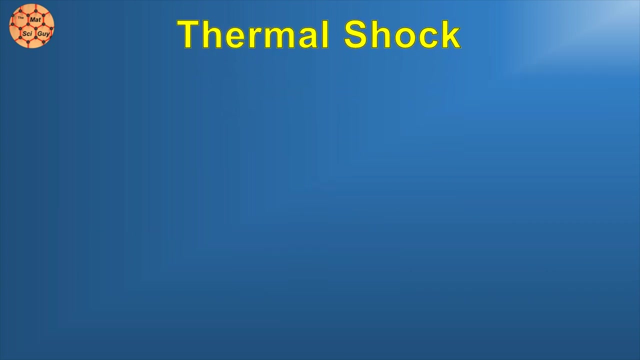 Even if you aren't a material science aficionado, you might know the name Pyrex. It's a common sight on kitchen glassware and it's famous for being able to withstand thermal shock. Thermal shock itself is pretty intuitive. Materials tend to expand when heated. If the 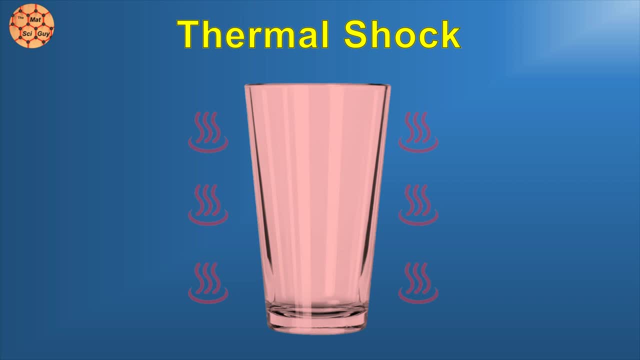 heating is used to heat the glassware, it will expand when heated. If the heating is used to uniform throughout the material, it usually isn't a problem. But if you have a sudden temperature change, obviously different parts of the material will be at different temperatures This causes. 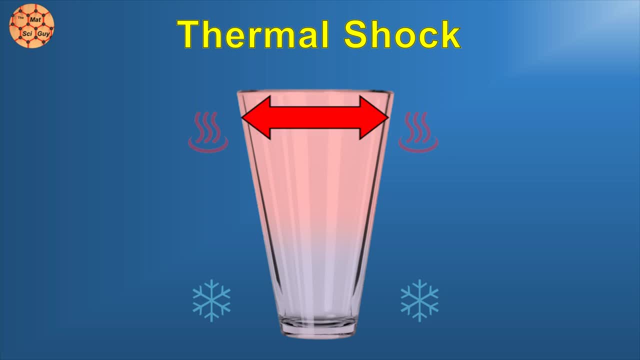 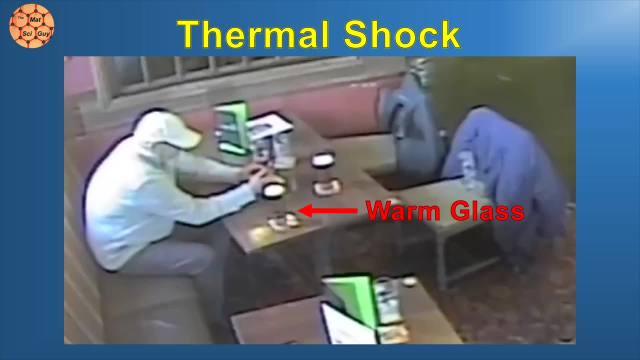 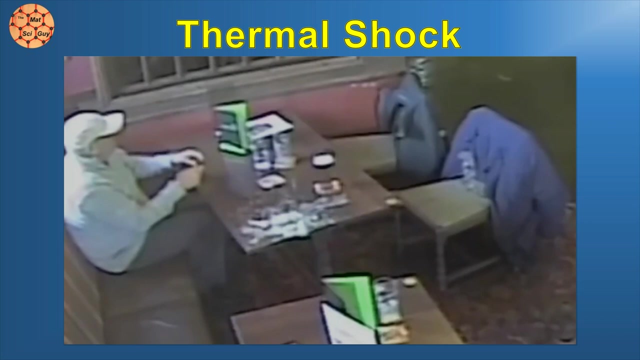 huge internal stress, as the hot parts want to expand but the cool parts don't, And eventually this can lead to catastrophic failure. If we want to make a glass that is resistant to thermal shock, we need to make sure that the heating is on. If we want to make a glass that 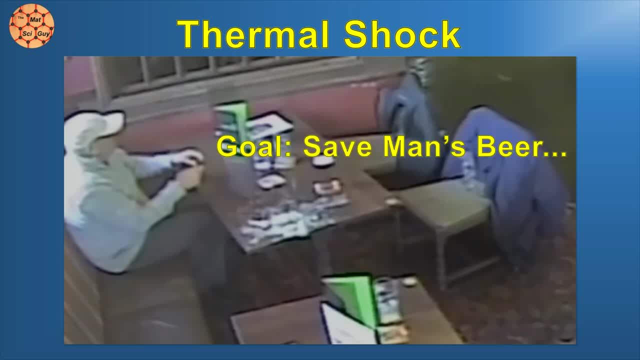 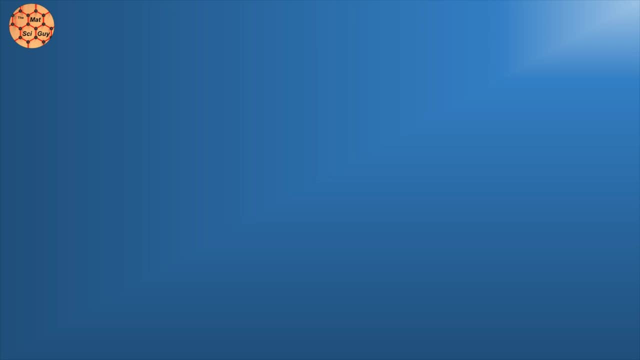 is resistant to thermal shock. we need to make it expand less when it heats up, And the material science behind how we can do so is pretty interesting. Let's start at square one. Why do most materials expand when heated? The easiest way to visualize it is to consider just two atoms. 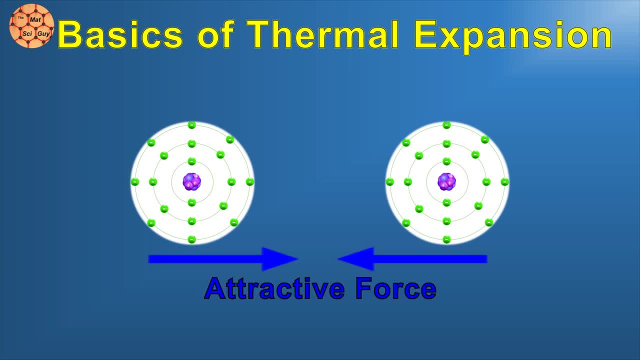 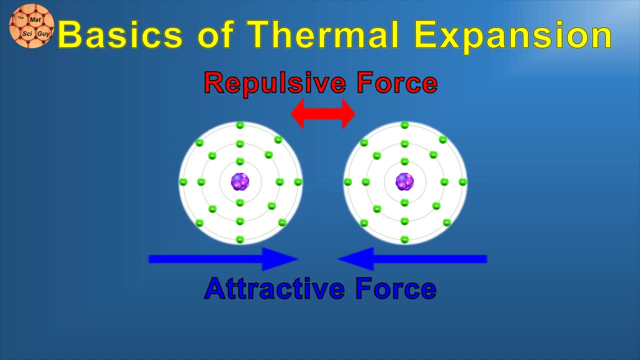 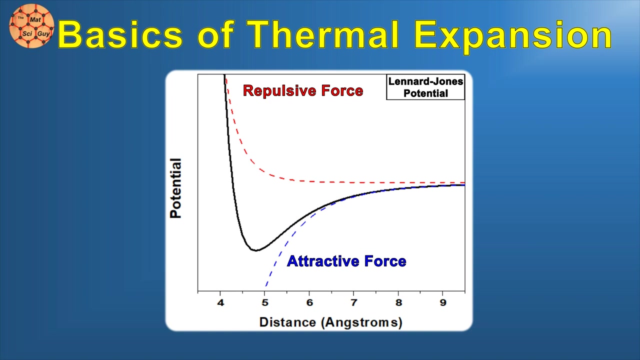 There's a relatively long-range attractive force that wants these atoms to be closer and a repulsive force that arises once electrons get close to overlapping. In the Leonard-Jones potential, a basic model of this, the repulsive force naturally falls off much more quickly with distance than the attractive force. 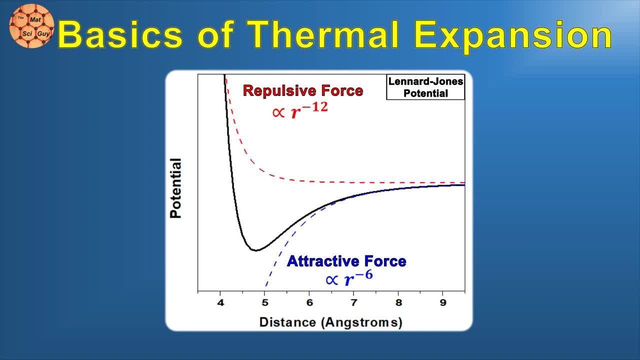 so the sum of forces forms this sort of well shape. An atom in equilibrium will tend to sit here, because it's where the attractive and repulsive forces are equal. This distance is the bond length. If we add some energy in the form of heat, we're basically moving the heat. 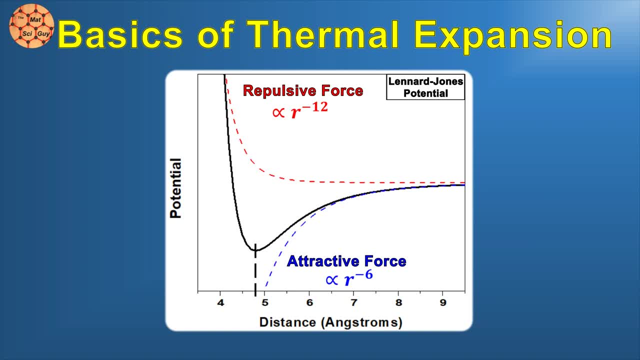 upwards in this. well, If it were symmetrically shaped, this wouldn't affect the bond length. The extra movement due to thermal energy can be in either direction, But remember that the repulsive force is a much steeper curve. This means that as we add energy, the average position 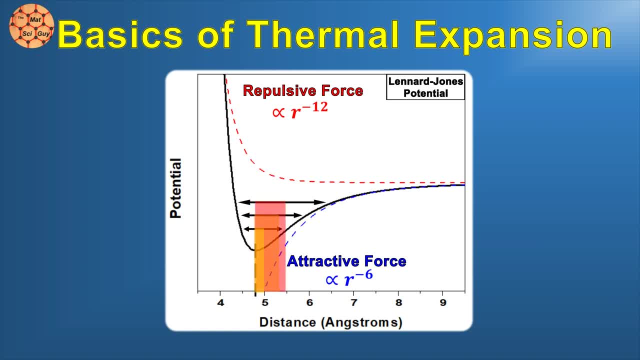 of this atom tends to be farther away from its neighbor. At this point I should mention that the Leonard-Jones potential isn't a real mathematical description of the forces involved and it comes with several caveats. but this principle of a mismatch between repulsive 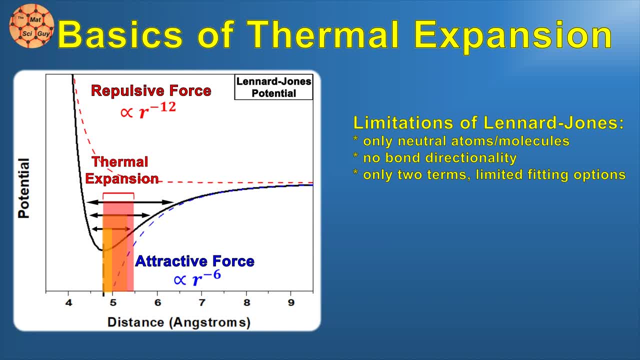 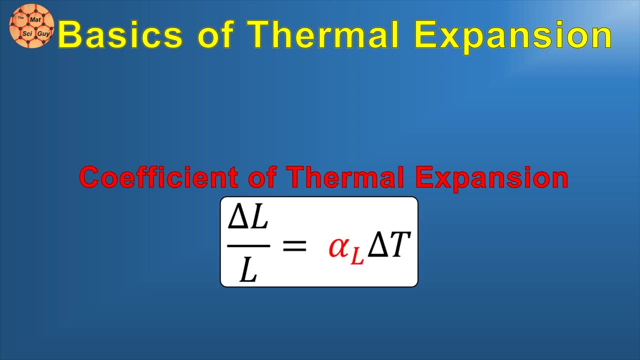 and attractive forces in the bond is useful for visualization purposes, and we can use this model to understand a very real trend in thermal expansion. How much a material expands when it's heated is usually expressed in terms of the coefficient of thermal expansion, or CTE. 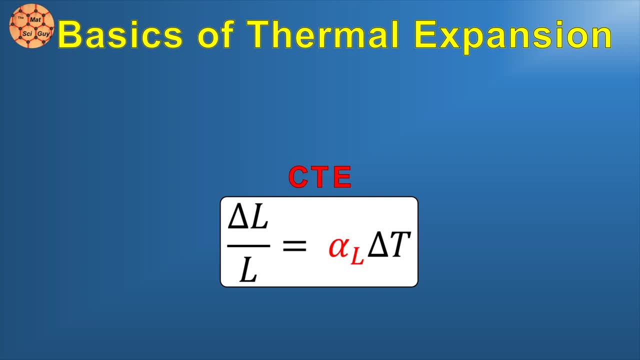 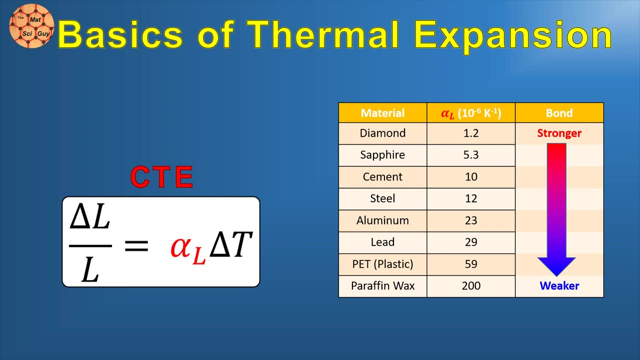 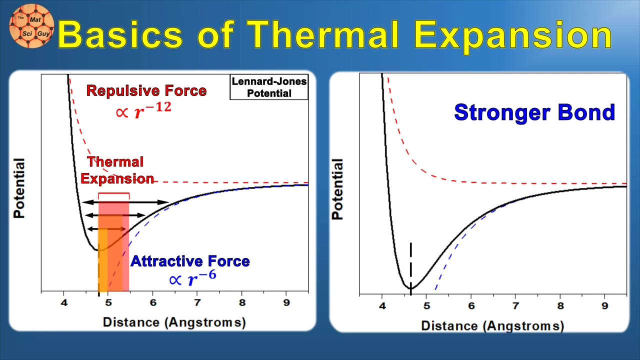 There are many factors that affect a certain material's CTE, but one obvious pattern is that materials with stronger bonds tend to expand less. This can be easily understood in this model, since a stronger attractive force essentially means a deeper and more symmetric well, If we assume that the repulsive force is the same, 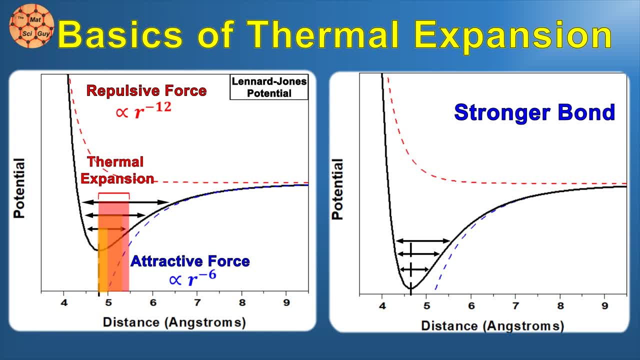 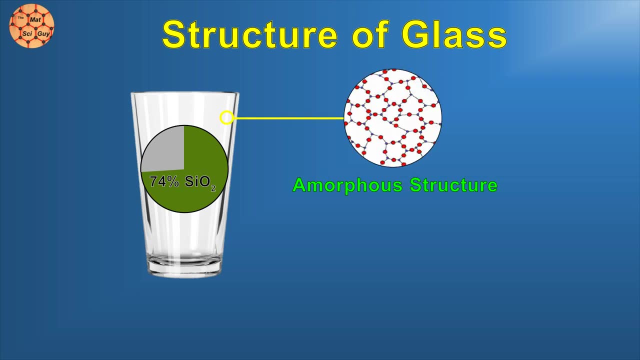 increasing the attractive force basically locks this atom into a tighter position, meaning less expansion with temperature. Now let's apply these concepts to our model. Glass is mostly silicon oxide- SiO2, arranged in an amorphous network. These bonds are very strong and actually this amorphous structure tends to expand. 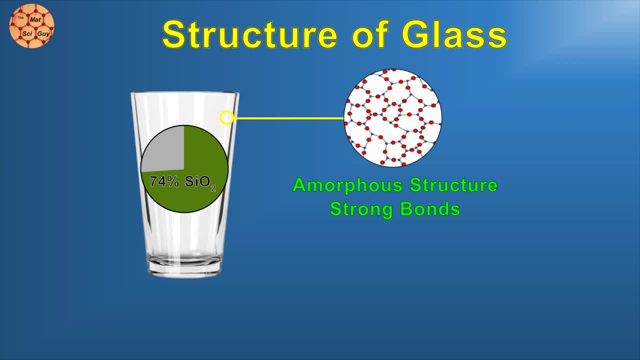 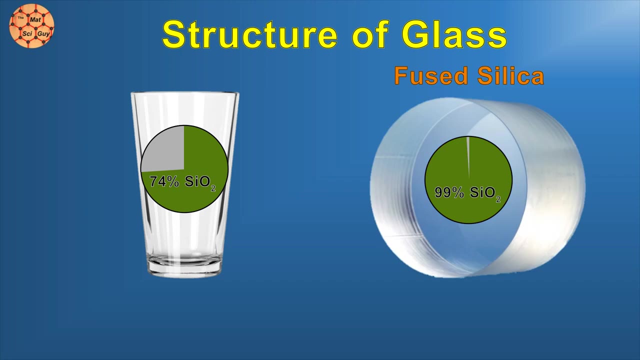 less than crystalline ones of the same composition. At first, this seems like a recipe for a material with a very low CTE, but the problem is that glass isn't pure SiO2.. Pure SiO2 glass is known as fused silica, and it's an outstanding material. 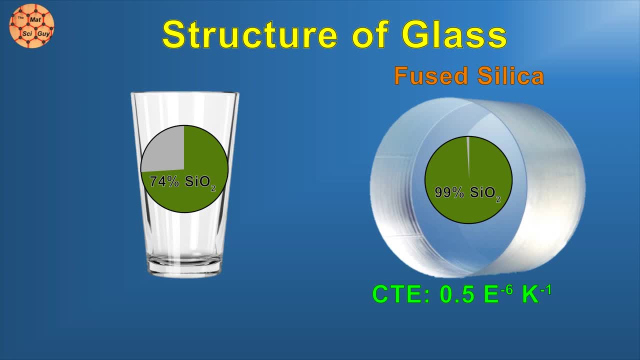 The CTE is extremely low, like we'd expect, and it's very chemically and mechanically stable. The problem is that it requires extremely high temperatures to melt and process. To make glass easier to shape at lower temperatures, other oxides are added. 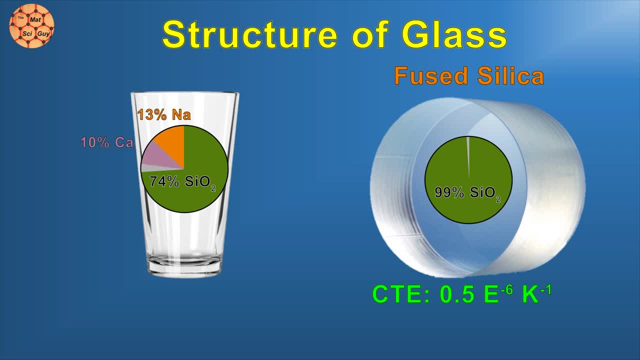 most notably ones like sodium and calcium. This makes soda-lime glass the stuff that you see in windows and the vast majority of glass products in general. The CTE of soda-lime glass is over 10 times higher than fused silica, and to understand why, we need a bit of background on how the bonding works in this system. 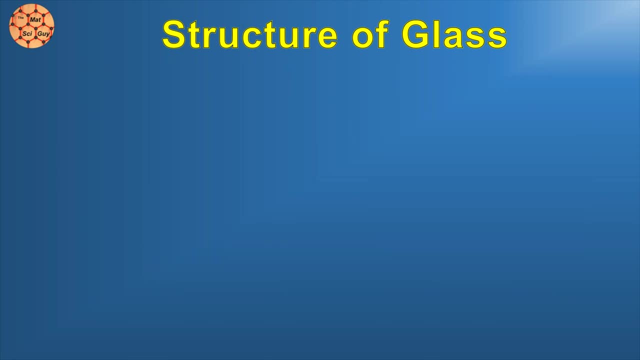 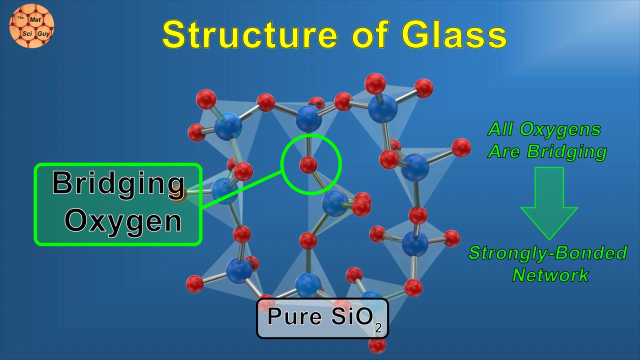 You see, in pure SiO2, the atomic structure is this sort of tetrahedra, with each silicon atom bonded to four oxygen atoms. Oxygen can bind with two silicon atoms, bridging them and making everything a solidly bonded network. This can almost be thought of as a single giant molecule. 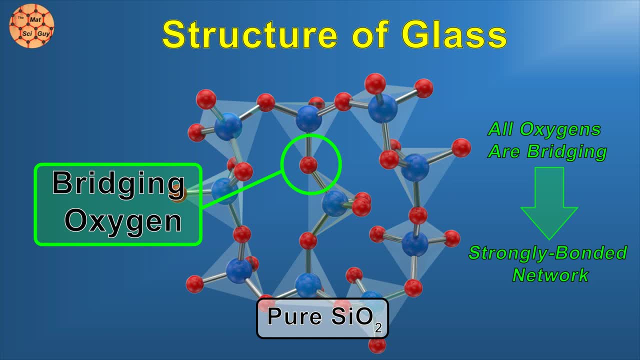 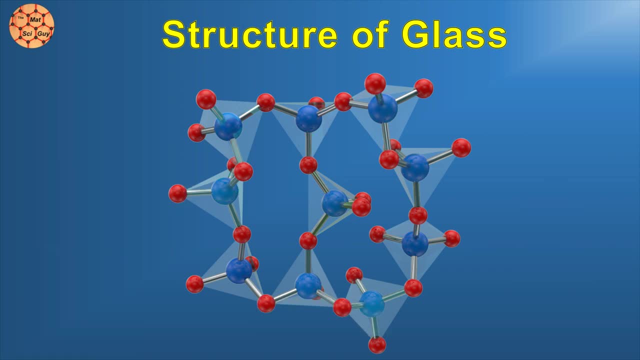 Everything is well connected with very strong bonds, but when we introduce an additive like sodium, our nice network starts to degrade. As an alkali metal, sodium really wants to lose an electron, and only one electron. When that happens in our nice network of silica, 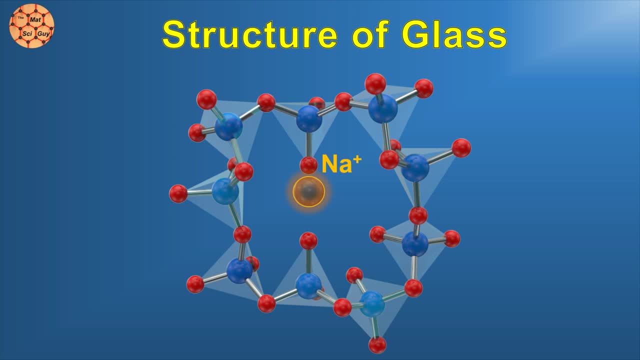 it drops off that extra electron and creates an oxygen that is no longer bridging silicon atoms, or any atoms for that matter. The creation of these non-bridging oxygens leads to a sharp decrease in network connectivity and makes the CTE increase significantly as more alkali or alkali-earth. 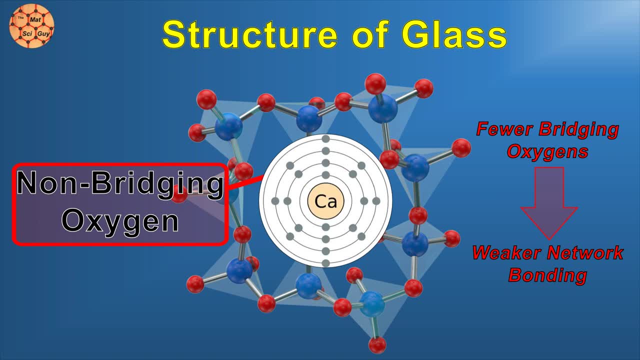 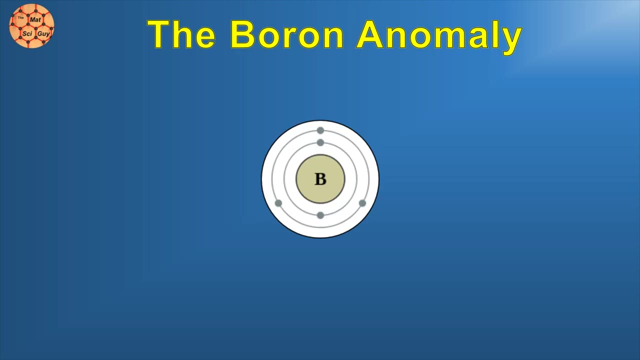 oxides are added. Calcium functions in a similar way, with the only difference being that it creates two non-bridging oxygens per atom. Now let's introduce boron. Boron is a bit of a weird character in this whole saga because at first glance he seems to function kind of like the other. 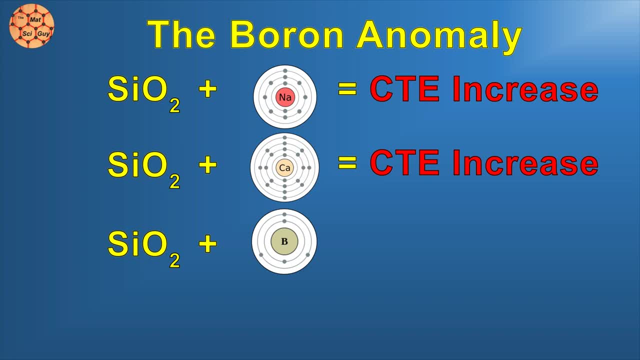 additives. If you add boron to pure silica glass, the CTE increases. Not much to see here. The interesting thing happens when you add boron to a glass that contains alkali-ions like sodium. The CTE decreases dramatically all the way to less than half that of soda-lime glass. 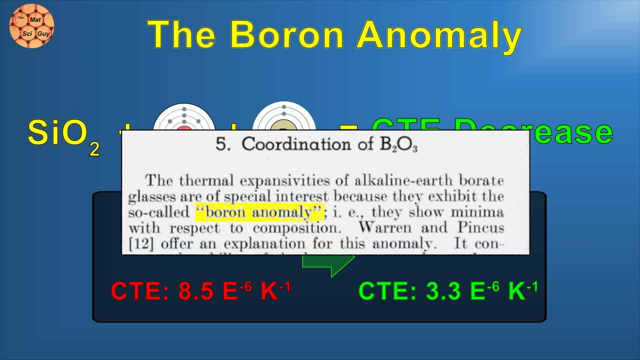 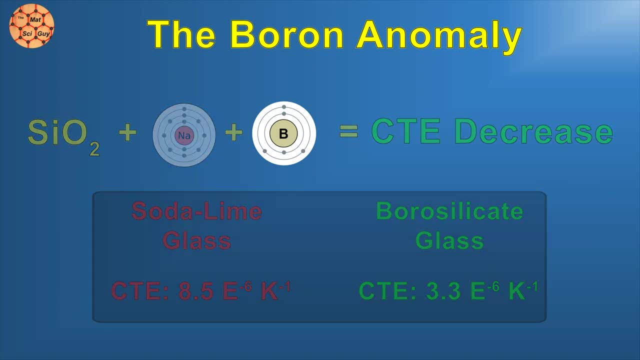 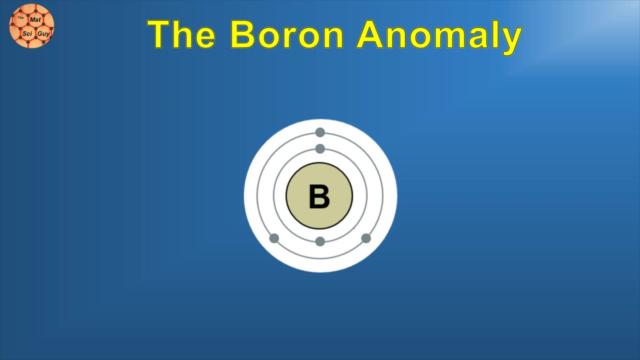 This was dubbed the Boron Anomaly, and scientists initially weren't sure of exactly why this happened. What was later discovered is that boron can actually have two different structures in this system. Normally, boron is an alkali. It likes to have a coordination number of 3, which makes sense, since it has 3 valence electrons to give. 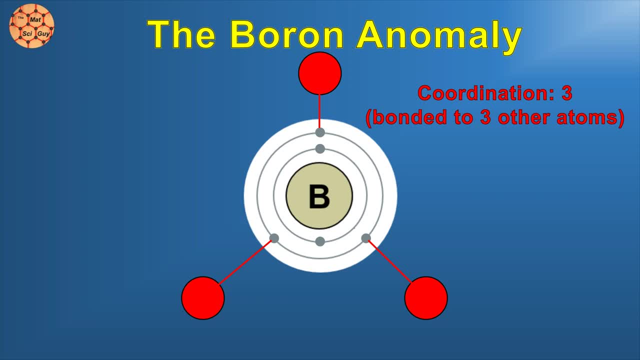 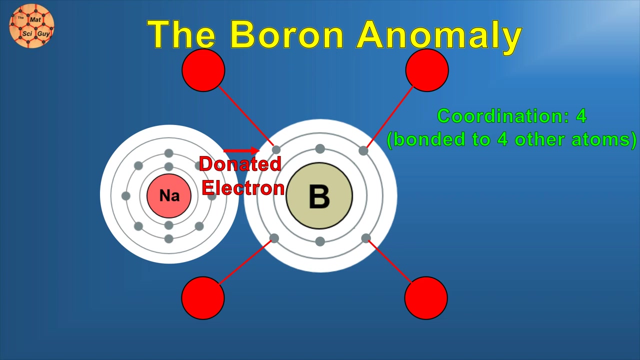 This ends up disturbing the silica network and not helping reduce our CTE at all. However, if we add sodium or any other alkali metal, boron can actually have a coordination number of 4.. This is the big secret to the low CTE of borosilicate glass. 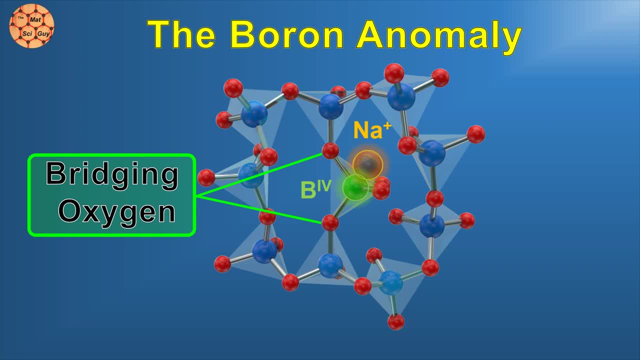 Not only is the boron now better connected in the network, but the sodium atom is now no longer free to create non-bridging oxygens. Network connectivity is restored and we now have a glass that is less prone to thermal shock, while still being fairly easy to process at reasonable temperatures. 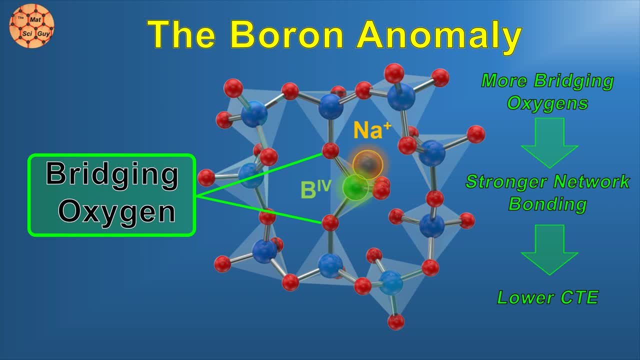 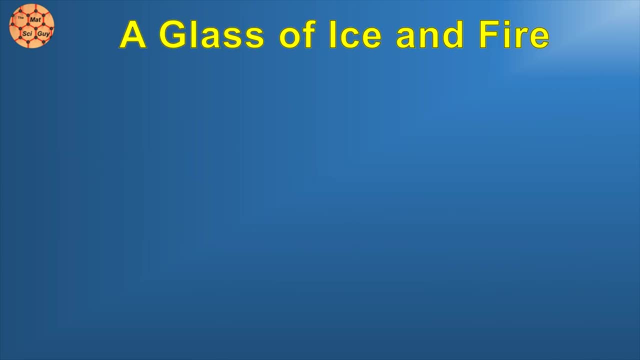 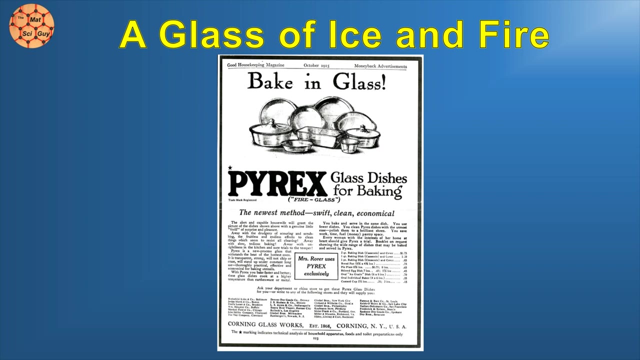 Borosilicate glass has been available commercially for over 100 years now, and its impact has been felt everywhere. Glassmaker Corning originally marketed its borosilicate glassware under the name of Pyrex, and it quickly became a common sight in kitchens everywhere. 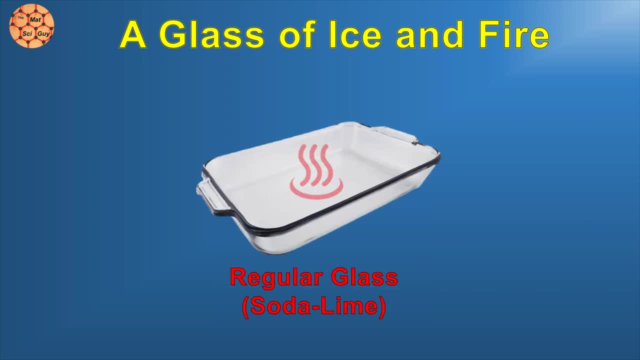 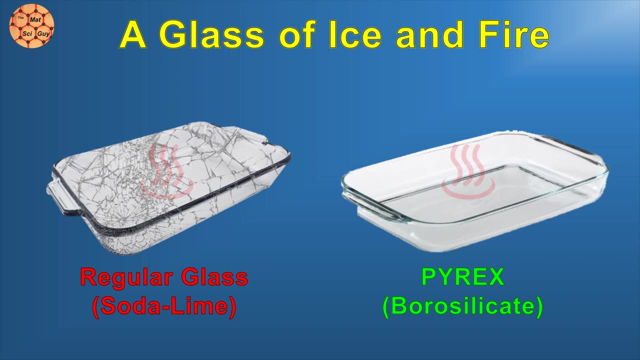 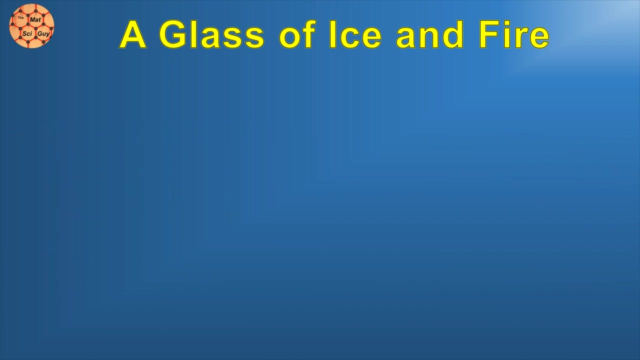 Unlike regular soda lime glass, which would tend to shatter when suddenly heated or cooled, Pyrex was stable enough to handle all of the duties of ceramic or metal kitchen items. In addition to consumer glassware, borosilicate made a big impact in scientific labs. 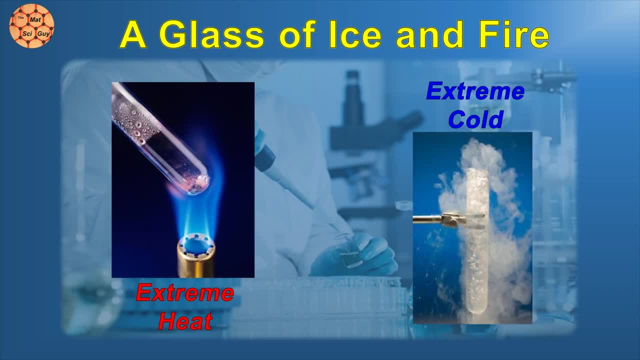 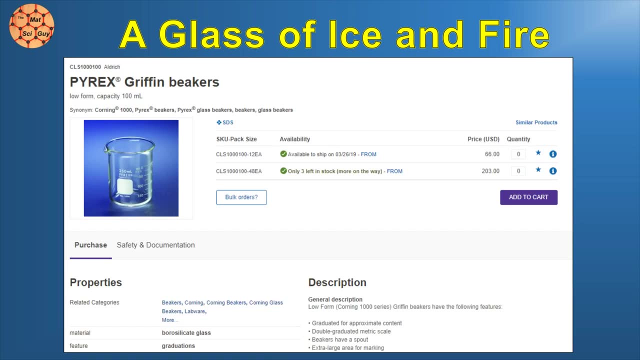 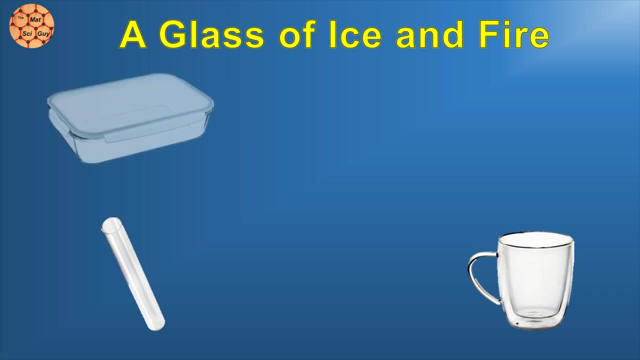 where glassware is often subjected to extreme temperatures. Borosilicate glass sold under both Pyrex and other names was incredibly useful there, and it remains the standard for scientific glassware today. Overall, countless borosilicate products have been sold, but the classic Pyrex measuring cups with the distinct red markings are probably the most iconic. 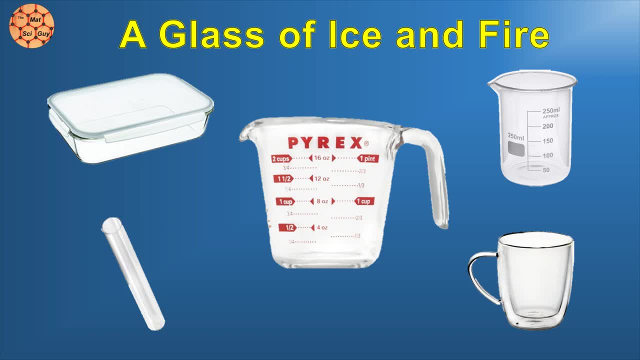 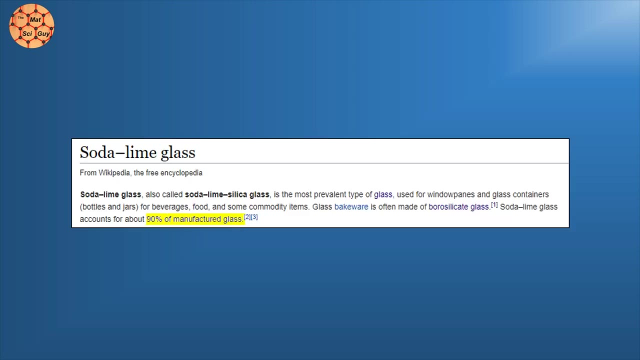 The name Pyrex became so well-known that some still use it as a term to mean diarrhoea- borosilicate glass in general. So if it's so great, why isn't everything borosilicate glass? Why are most of our glass products still just the regular soda lime glass that's prone to thermal? 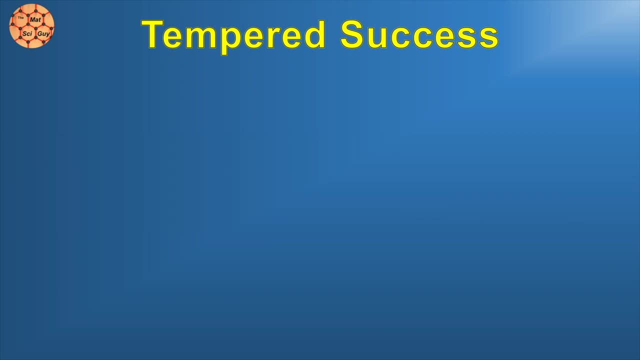 shock. Well, one reason is simply price. Borosilicate glass is significantly more expensive and it's just not worth it in applications where resistance to thermal shock isn't required. Another disadvantage of borosilicate glass is that a low CTE is a bit of a double-edged sword. 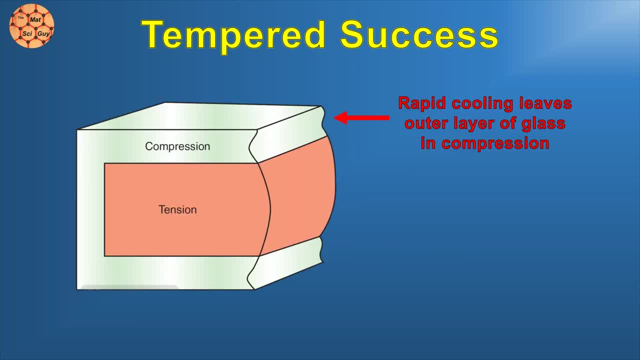 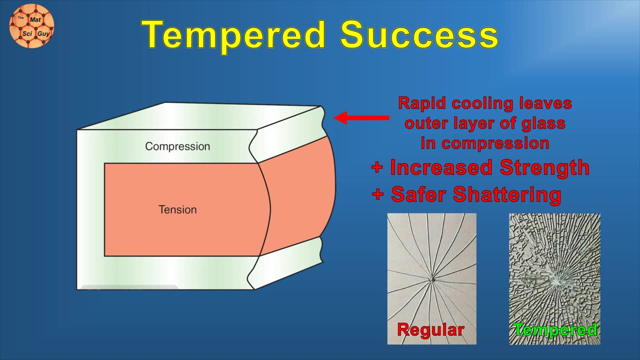 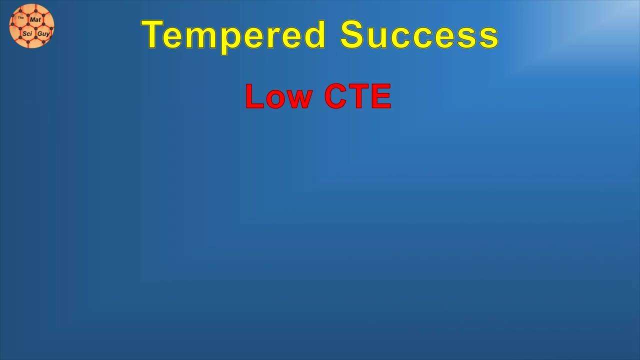 Tempered glass is soda lime glass that has been rapidly cooled. This makes the glass mechanically stronger and makes it shatter in a much safer way, forming smooth chunks rather than the sharp pieces like non-tempered glass. The low CTE of borosilicate glass means that this heating-cooling 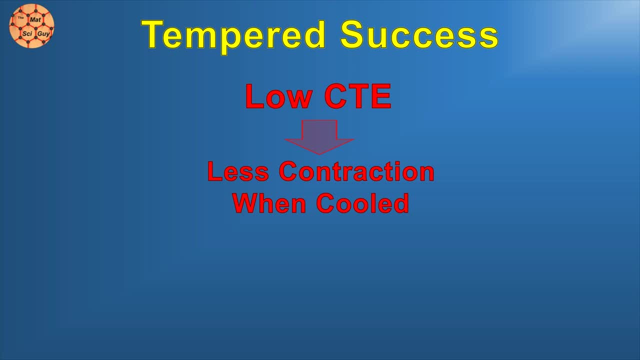 process is not as effective as it used to be, So if you're a borosilicate glass lover, can't really produce the same effect and, as a result, it can't be tempered in the same way, Despite becoming synonymous with borosilicate glass. 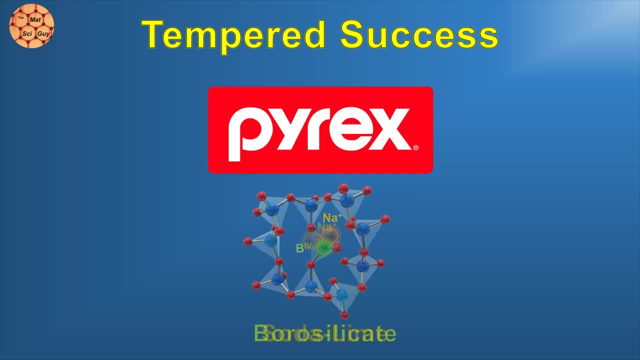 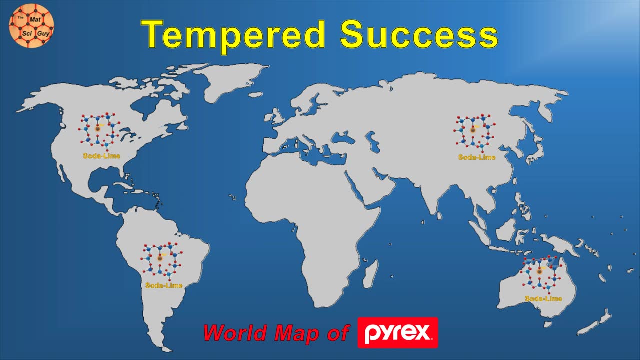 many things sold under the Pyrex name are now just tempered soda lime glass. The company which makes Pyrex in North America has been using exclusively tempered glass since 1998, but in Europe and some other regions Pyrex is still true borosilicate glass. 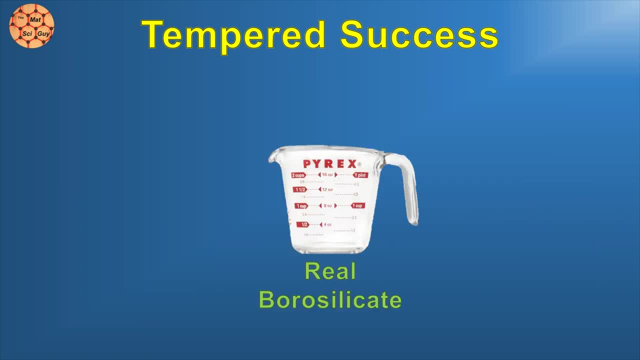 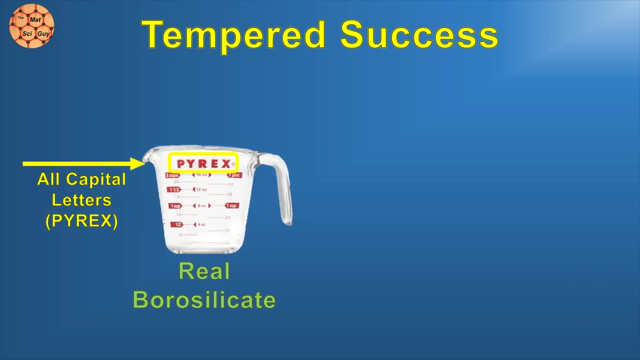 Even though it's the same name. the real borosilicate ones still sold outside of North America are distinguished by all capital letters. Tempered glass bearing the Pyrex name is all lowercase and it often has a more bluish tint. Of course, the parent company claims that their 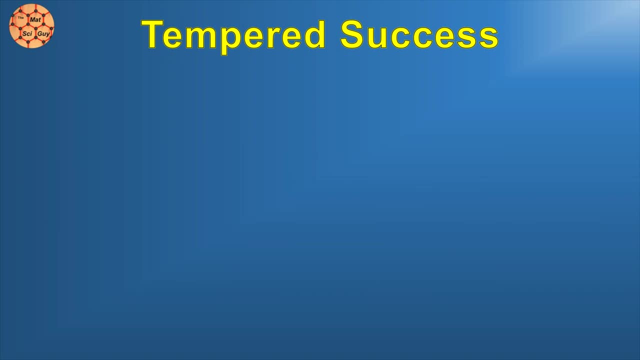 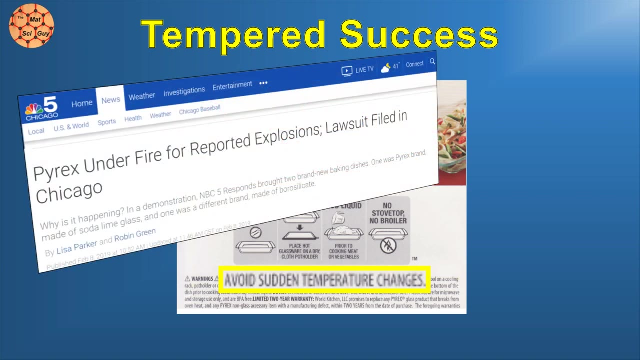 tempered glass is safe for most kitchen use, but it's still not as resistant to thermal shock as the original borosilicate variety, And there's even a lawsuit related to the company's use of Pyrex bakeware exploding in ovens. It's a bit sad to see a brand name that once meant a truly 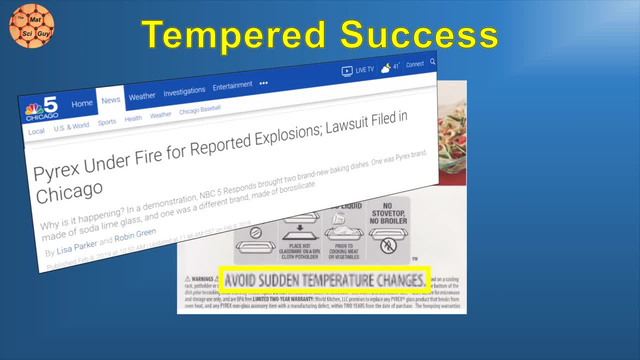 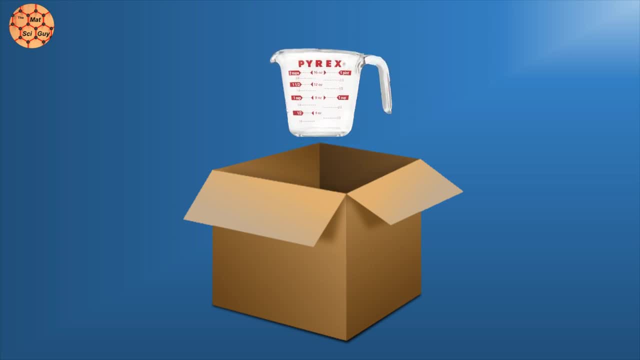 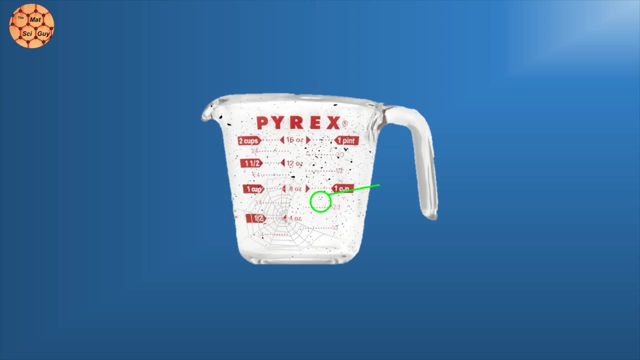 special type of glass being reduced to this. So if you live in North America and you find some really old Pyrex glassware in your kitchen, don't be so quick to throw it out. It might be a bit dusty and worn, but you're holding something truly unique and special. It's a material that 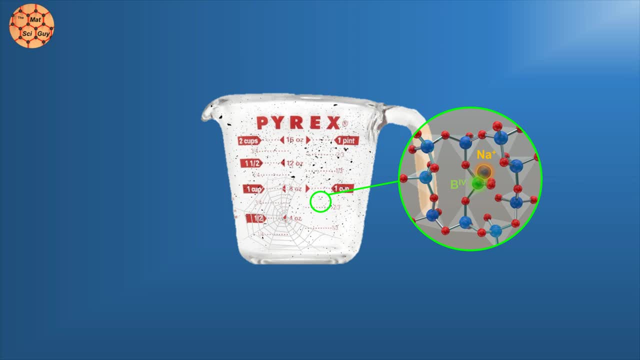 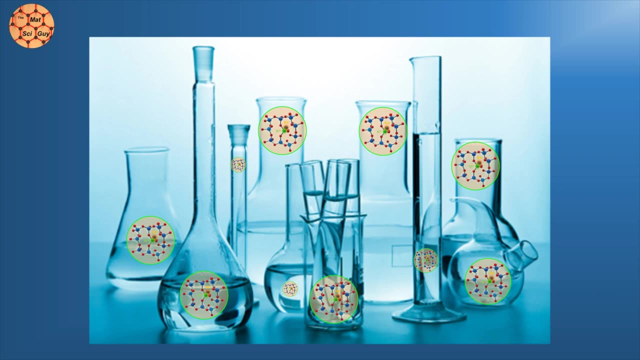 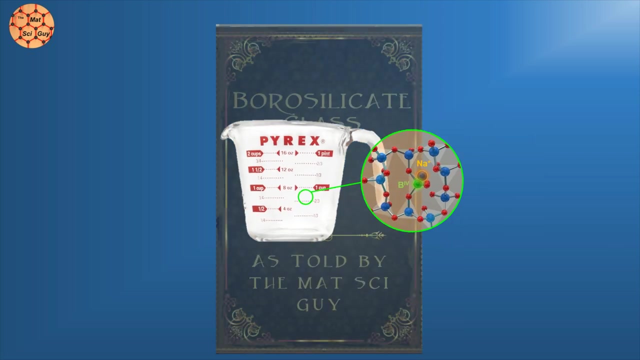 revolutionized glass in general, And its impact can still be seen in scientific laboratories around the world, even as its popularity wanes in the consumer market. That old measuring cup can last for many more years if you take good care of it, and you too can be part of the story of borosilicate glass. 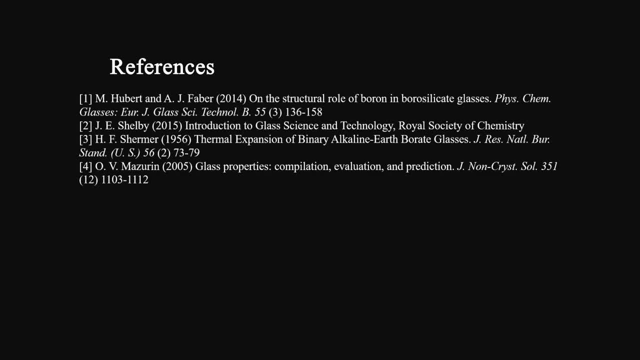 Subtitles by the Amaraorg community.